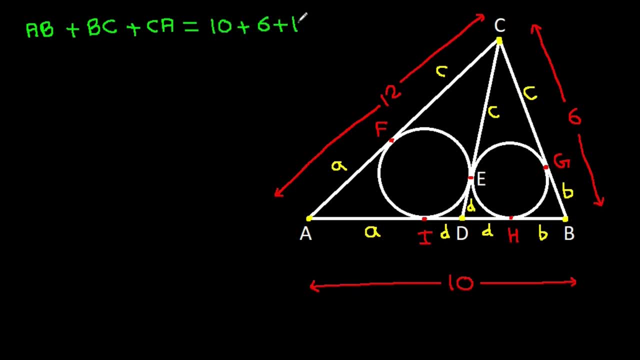 Let's take essential function now by the second quarter. So now let's iterate all chains. Let's say AB miniинов Bianco I- And since here he is said to be one of So camino- is independent, then AL this whole thing remains as this. 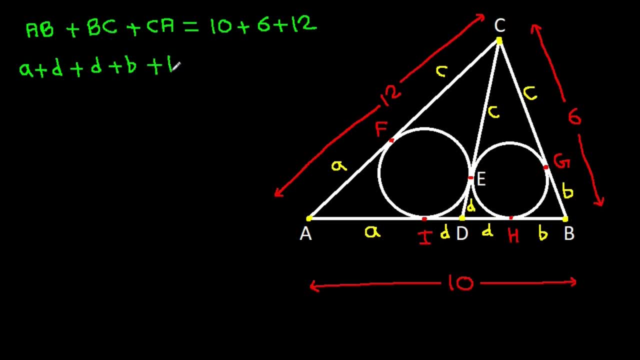 So at this COMB sini este deome distinguished. bc, it is b plus c plus ca, it is c plus a, that is equal to 10 plus 6 plus 12, it will be 28, and a plus a is 2a plus b plus b is 2b plus c plus c is 2c plus d plus d is 2d, it is 28. 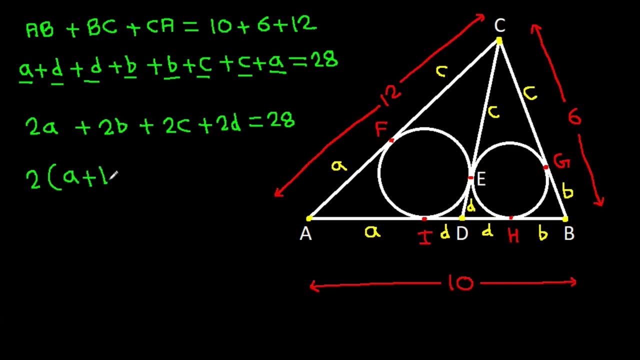 and it is 2 times a plus b plus c plus d is 28. and it is 2 times a plus b plus c plus d is 28. so a plus b plus c plus d, it will be equal to 28 by 2. so a plus b plus c plus d, it is equal to 14. 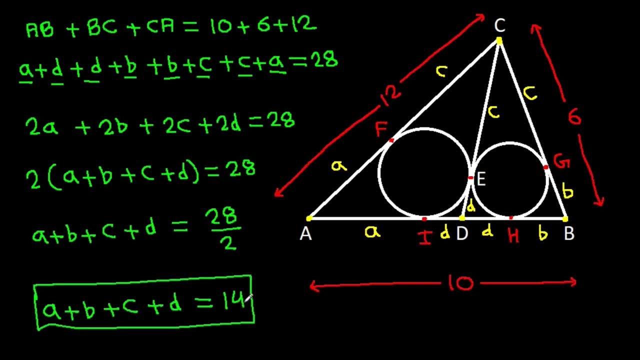 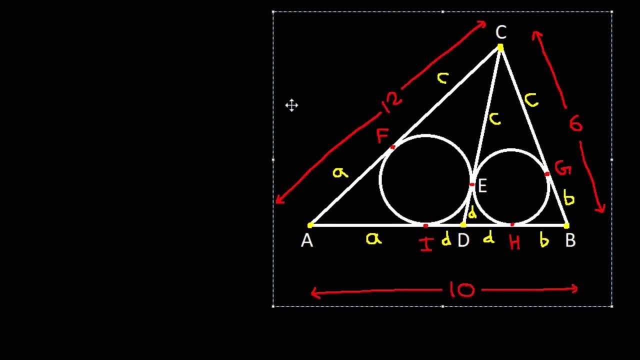 and we have a plus b plus c plus d is 14, and now ac it is equal to a plus c, that is 12. so b plus d it will be equal to a plus b plus c plus d is 14, and now ac it is equal to a plus c, that is 12. 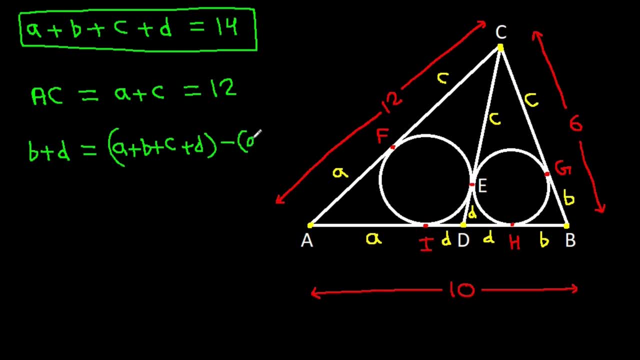 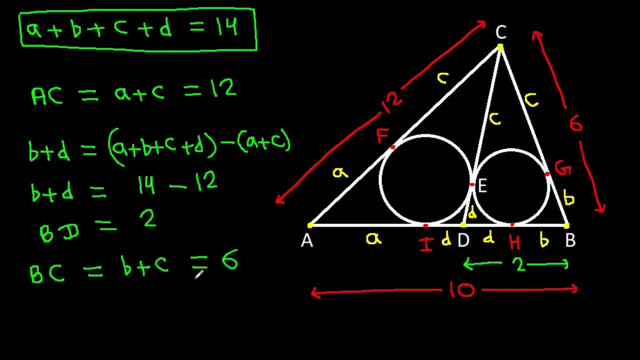 is b plus c, that is 6.. So a plus d, it will be equal to a plus b plus c plus d minus b plus c, And a plus d, it is ad. it is equal to 14 minus 6, that will be 8.. So ad it. 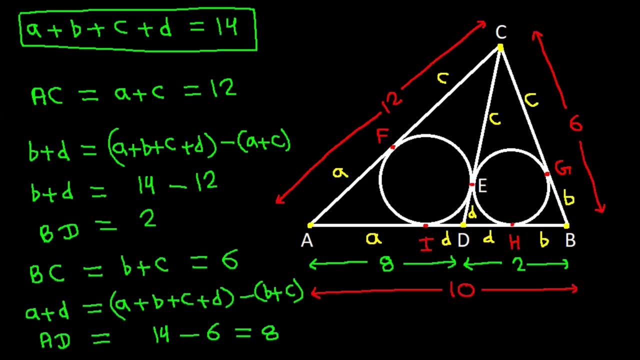 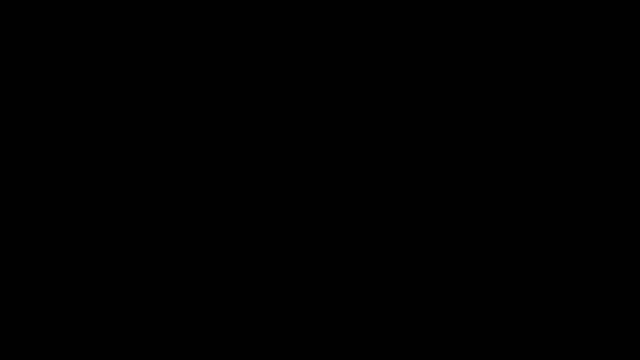 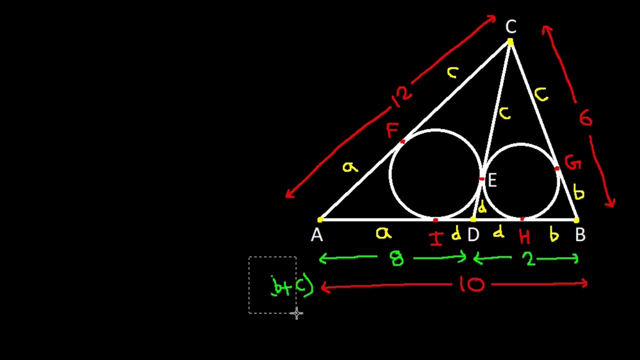 is 8.. And now from Stuart's theorem, in any triangle- a, b, c and d, if ab is b, ac is c and bc is a and bd is m, cd is n and ad is b. 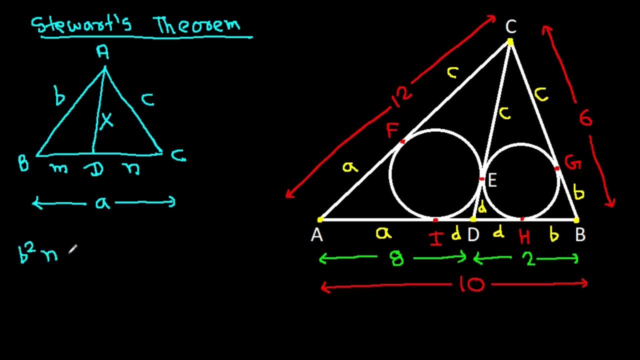 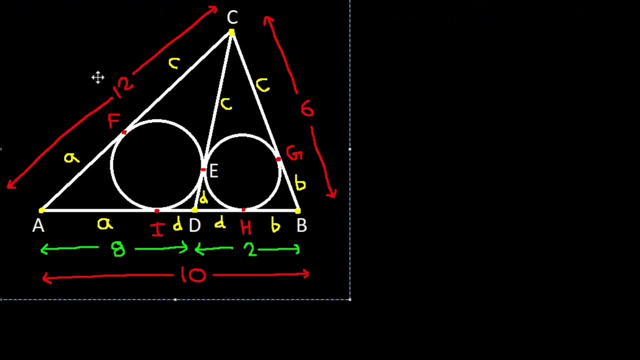 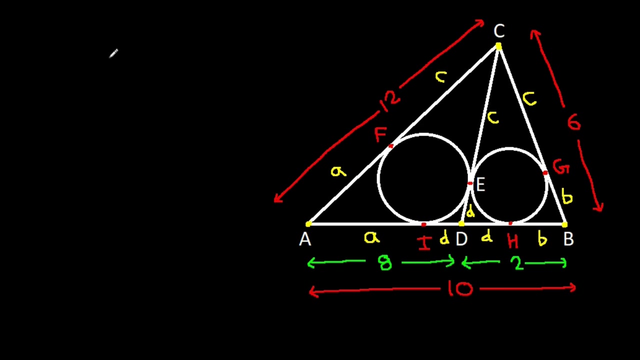 Then b square n minus c square m, it will be equal to a times mn minus x square. And here interangle abc. it is a, b, c and d. We have ab is 10,, ad is 8, bd is 2, and ac is 12,, bc is 6.. So 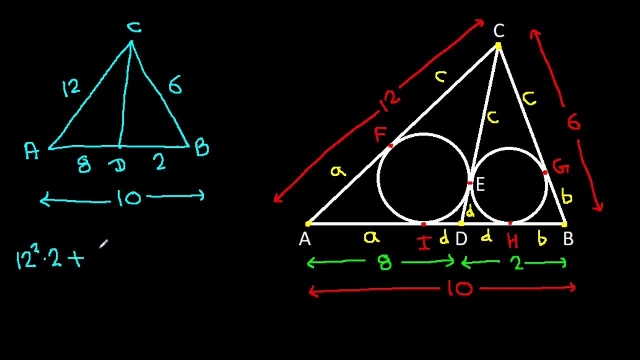 now by multiplying byまり with b, c. we need a connective denominator And credits is x square plus c square, then it becomes 144 times 2 plus cb, which equals Av. The question is: thanks if c is x?